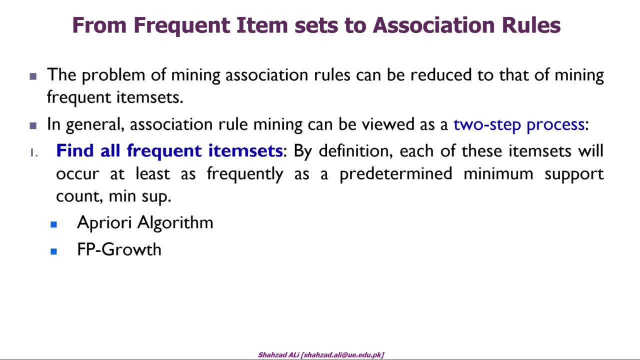 we have to mine frequent item sets from the you know transactional database and after mining frequent item sets we can generate association rules from those frequent item sets. so there are different algorithms for mining frequent item sets from transactional database, in which we have two very famous algorithms. the first one is a priori algorithm and the second 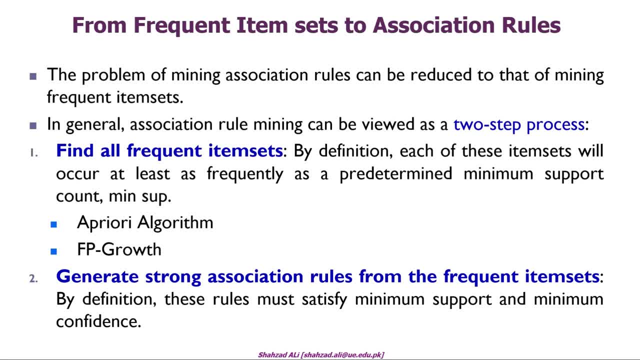 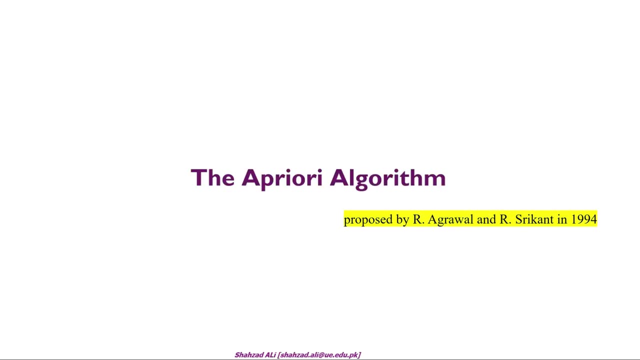 is FV growth algorithm or frequent pattern growth algorithm. after mining the frequent patterns using any of these algorithms, we will try to generate association rules from frequent item sets generated by a priori algorithm or frequent pattern growth algorithm. so in this lecture we will cover the a priori algorithm. so this a priori algorithm is proposed by Agarwal and Srikanth in. 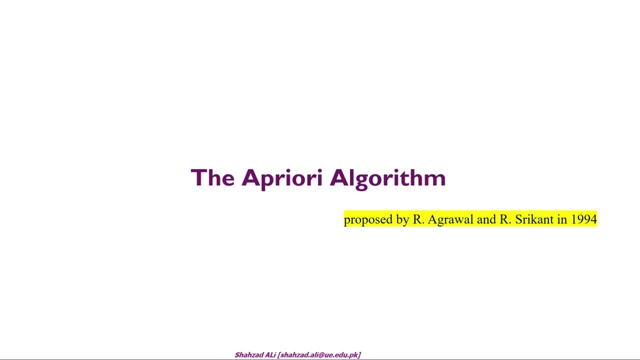 1994 for mining frequent item sets for Boolean classification. Boolean association rules in As94b. the name of the algorithm is as follows: is based on the fact that the algorithm uses pure knowledge of frequent item sets properties as well as as we shall see later. so a key concept in a prairie. 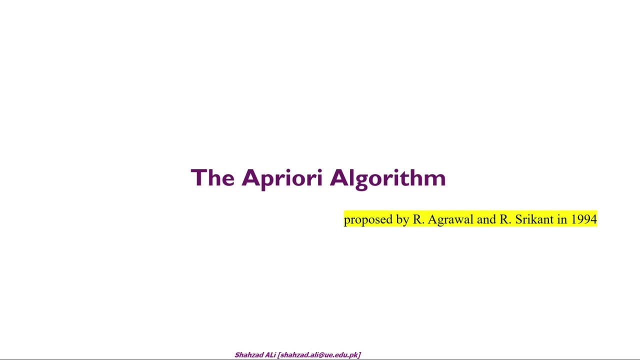 principle is to assume that all subsets of frequent item sets must be frequent and similarly, for any infrequent item sets, all of its superset superset must be infrequent. so this algorithm is at the first candidate generation and test approach for frequent pattern mining. it is a level wise, you know. candidate. 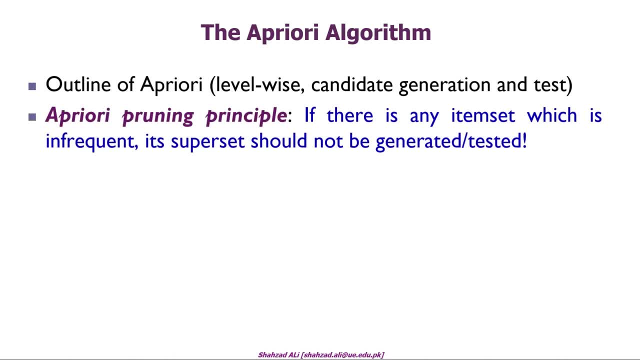 generation test approach. a prairie principle or a prairie pruning principle indicates that if there is any item set which is infrequent, its superset should not be generated or even tested. so a prairie principle can also be defined by another way, in another way that all non empty subsets of a frequent item set must also be frequent. 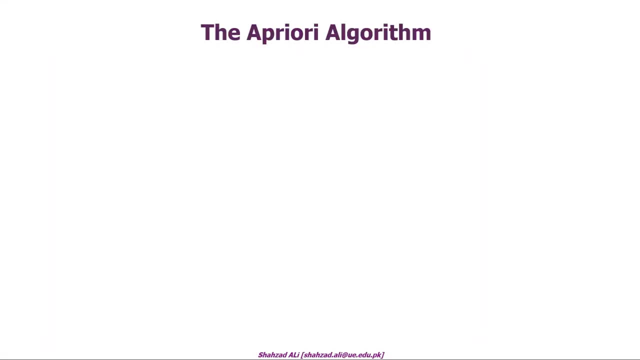 plus users release aCK value provided to the following persistent Guess Warren economics list and it 194. the algorithm of a prairie algorithm works as follows: initially, the first time, you just scan the database once to get frequent one item set. then taking this frequent one item set, 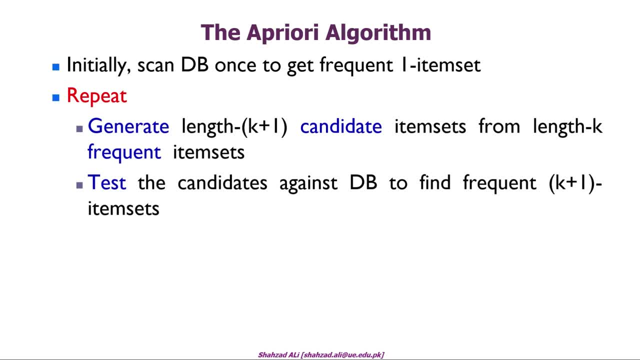 And at the kth iteration you are going to take a length k frequent item sets to generate length k plus 1 candidate item sets. So then you go against the database to test these candidates generated and to find the frequent k plus 1 item sets. 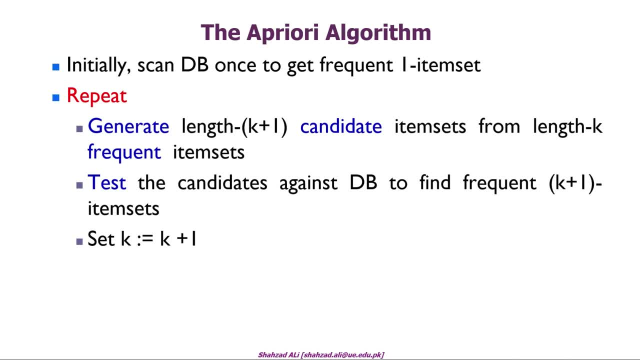 Okay, at every iterations you just set the k to k plus 1. So you can go on and on until no frequent item set will be generated or no candidate item sets can be generated. Okay, then, after you exit from the loop, you just return all the frequent item sets drive. That's the algorithm. 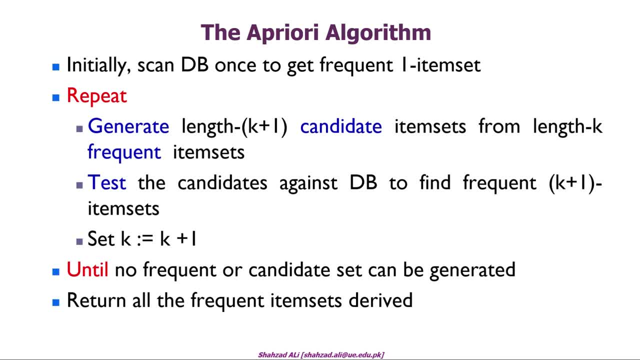 So, if we summarize this, a priori algorithm Is that at the first iteration, when we scan the database for the first time, we get the frequent item sets from that. Those frequent item sets are those that are fulfilling our minimum support count And remaining tooth sets that are less than minimum- you know, minimum support count, their occurrence or frequency- is discarded. 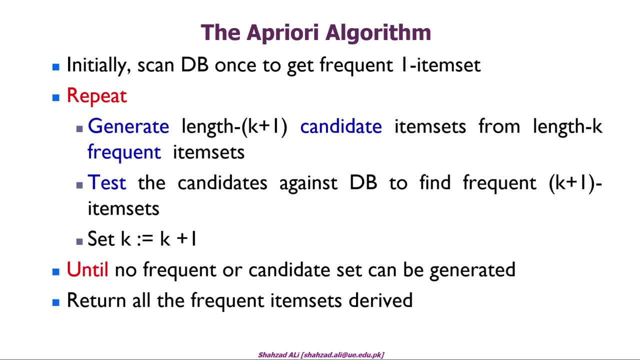 And then those frequent items. from frequent one item set we generate frequent two item set candidates. that how many candidates can be generated from that frequent one item set? so looking at those candidates, we again generate frequent two item set patterns. similarly, those who are less than minimum support threshold are discarded. 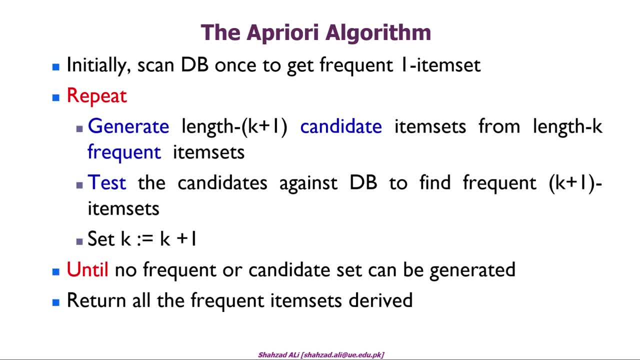 and those who are fulfilling minimum support threshold. we consider them as frequent two pattern. so from those two frequent pattern item sets we generate candidate three item sets and this process continues until any new frequent or candidate set is generated and at the end of this algorithm we return the frequent patterns or frequent item sets that we have derived. 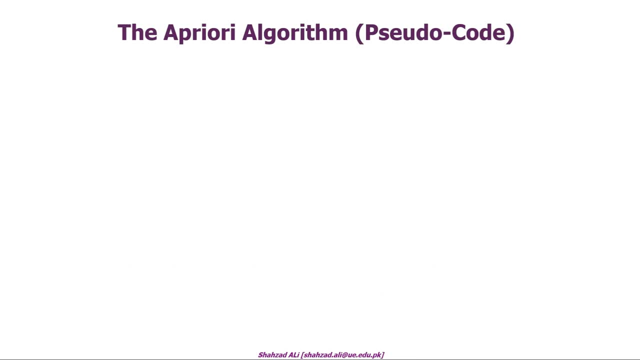 this was the overall algorithm, so let's look at the pseudocode of this algorithm. suppose we set C sub K to be the candidate item set of size K and F sub K is the frequent item set of size K. initially we just get a frequent one item set. 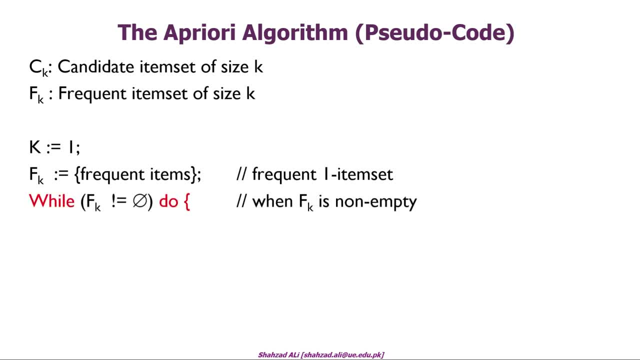 then we get into the loop. suppose the frequent K item set is not empty, then we use Kth frequent item set to generate K plus one candidate item set. then go against the database using the minimum support to see which K plus one candidate item sets are frequent. 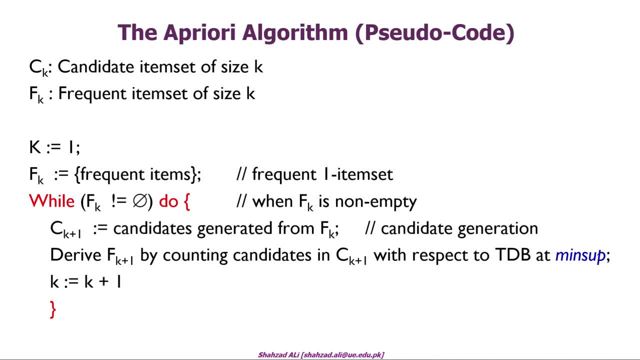 so, using those frequent K plus one item sets, we drive the frequent K plus one frequent item sets, then we reset the value of K to K plus one. until we get out of this loop we just return all the frequent K item sets for all the cases drive. 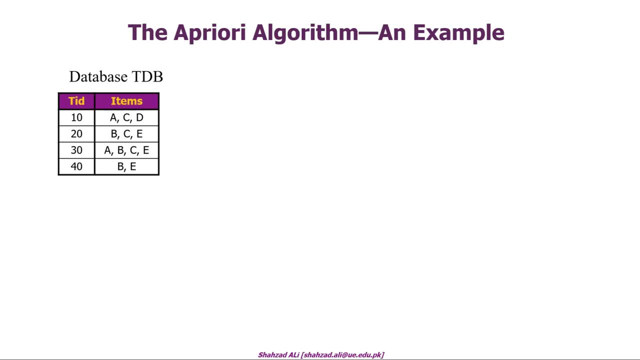 ok, so let's understand this working of the APRORI algorithm with an example. suppose we have a transactional database database, TDB, which contains 4 transactions and the transaction ID for these transactions is 10,, 20,, 30 and 40, and transaction 10 contains 3 items. 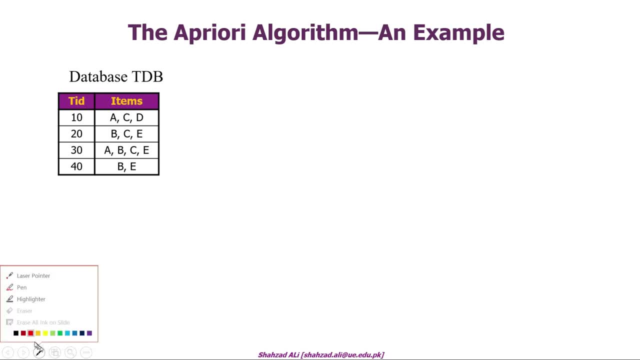 which is A, C and D. similarly, for transaction 20,, 30 and 40 we have different item sets in different transactions and suppose we set the minimum support threshold to 2, that means any item set that occurs 2 times or more than 2 times in these transactions. 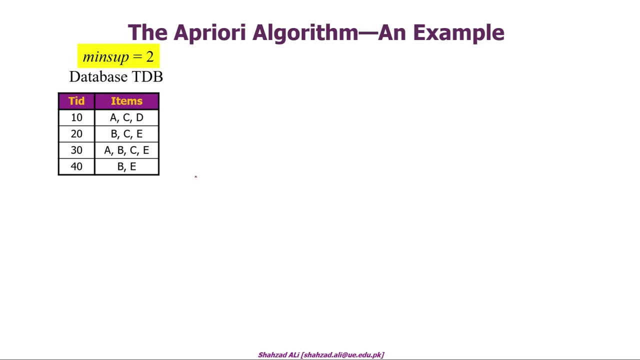 are frequent item sets, or in other words if any item set that appears less than 2 times is infrequent. so on the first scan of the database we get C1, candidate 1 item sets. that means A item set has support count of 2, as you can see in the transaction database. 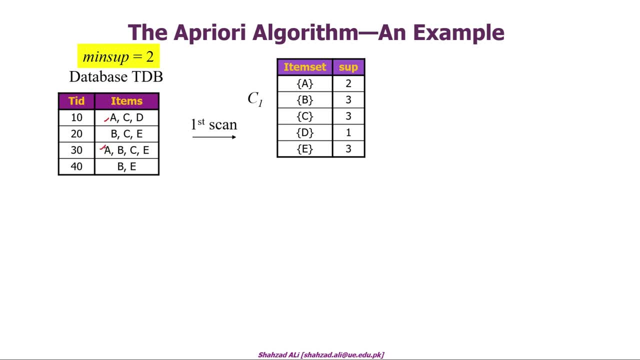 A, 1 and 2. A occurs only 2 times in the transaction database. similarly for item set B, it occurs 3 times. you can see here and here. similarly for item set C, D, which occurs only once, and transaction E, which occurs 3 times. 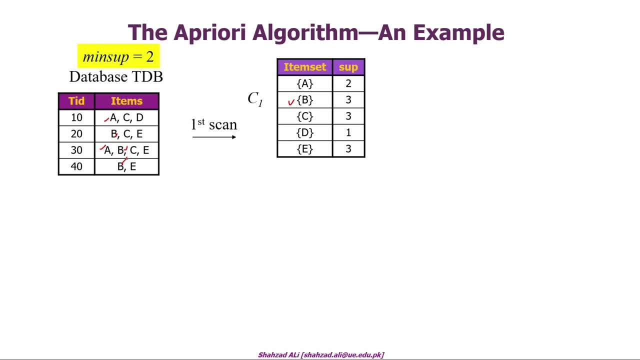 so, as we can see, the minimum support is 2. so this D item set is infrequent, so we discard D from the candidate item sets and our frequent one item set is A, B, C and E with the support count of 2, 3, 3 and 3 respectively. 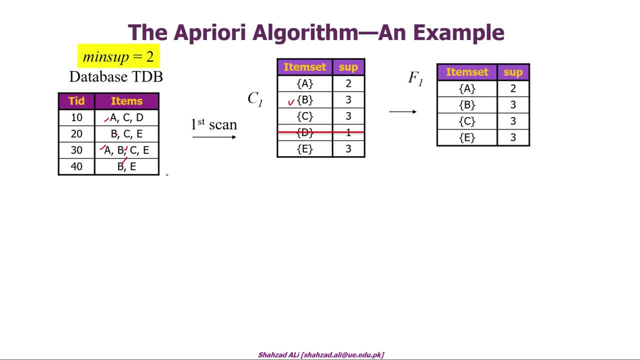 so using this frequent item set of length 1, we generate the candidate item sets of length 2. that means A, B, A C and A E, as you can see here in C2 table. similarly B, C, B E and C E. 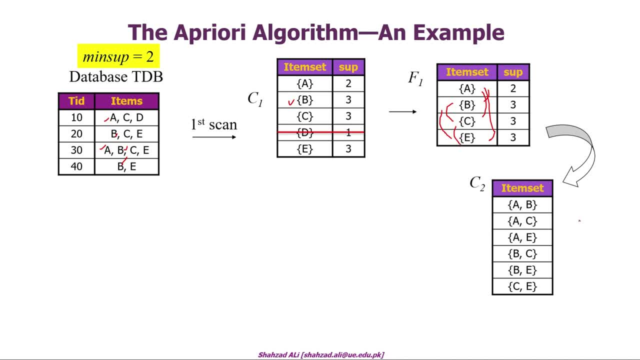 these are all candidate item sets of length 2. so we again go into the database, scan the database again and calculate their support count. like A- B, both items occur together only once in this transactional database, as A- B occurs in all in transactional ID 30. 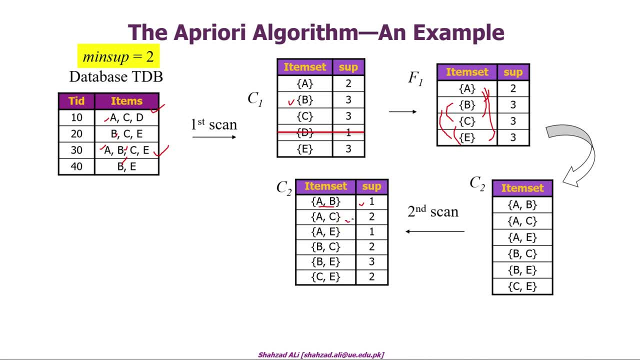 and similarly A- C transactions occur twice, like you can see here in transaction 10 and transaction 30 occur twice and similarly we have calculated the support count of each candidate item set of length 2. as you can see, A B and A E have support count of 1. 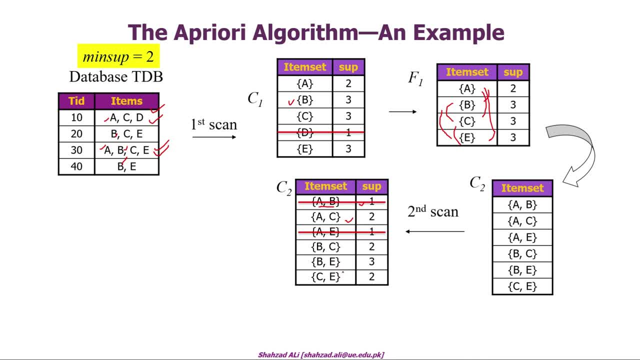 so that's why they they are removed from the frequent item set, and our frequent item set is A C, B, C, B E and C E, with the support count of 2, 2, 3 and 2 respectively. so we are so. 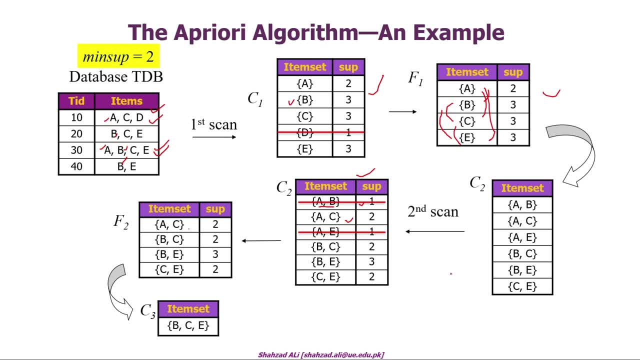 using this frequent 2 item set we generate frequent candidate item set of length 3, which is B, C, E. so remember this one. you people can see here is a big cut why? because you probably see A, C and B C as frequent. 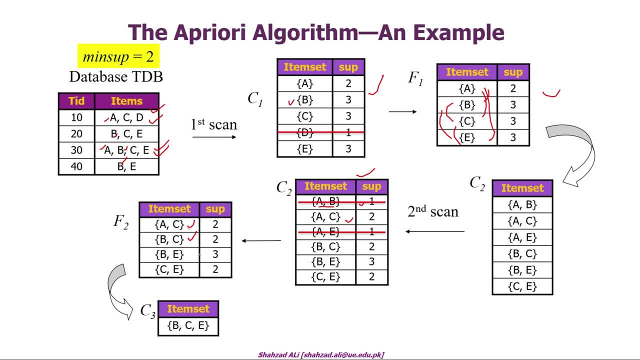 you might think A B C could be candidate item set of length 3, but A B is not frequent, as you see in this candidate item set of length 1. that's why we cannot consider A B C as frequent item set. 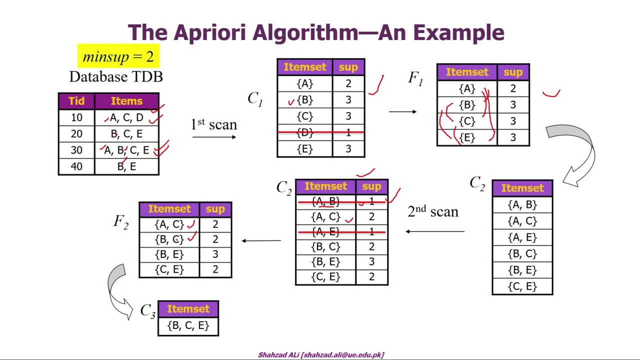 so you may consider that A, C and B C are frequent and then their super set is also frequent. so here is a problem: when we join these two item sets we get A, B C. so when we look into the candidate item set of length 2, 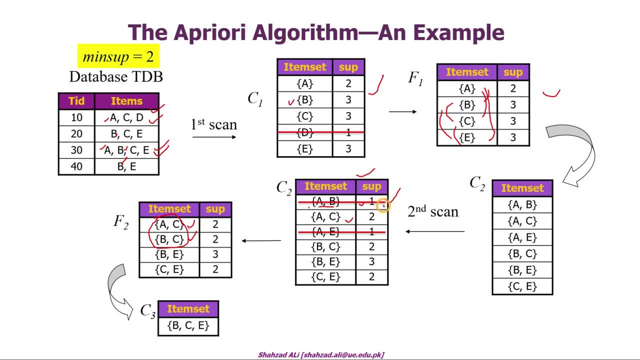 we see that A, B is removed as infrequent item set. that's why we cannot consider its super set as a frequent, so that's why it is removed, similarly others. so we only get B, C, E as candidate item set of length 3. 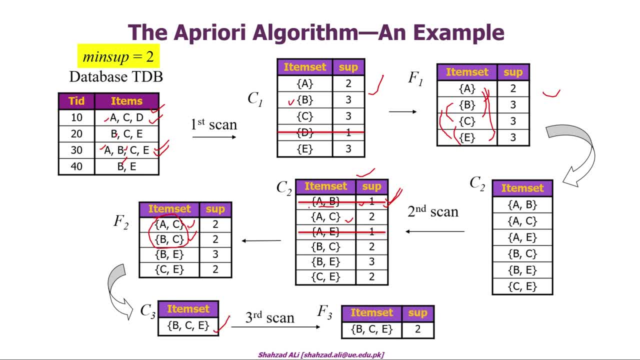 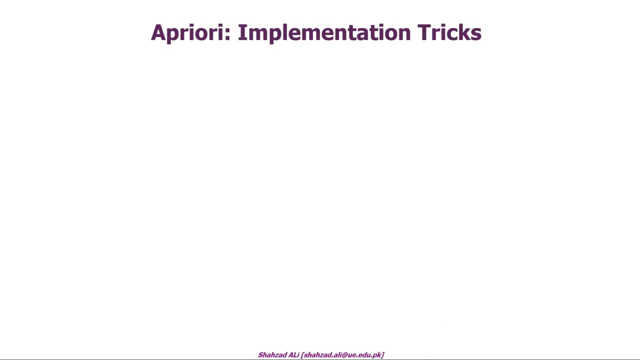 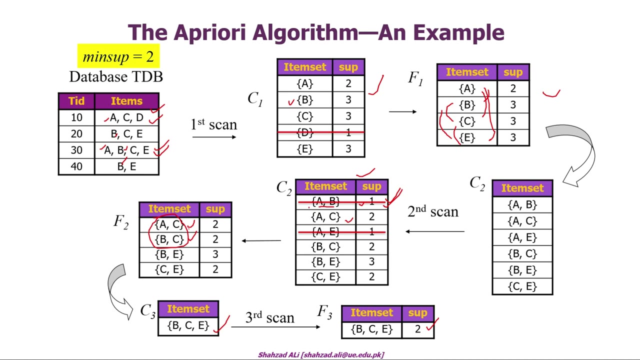 so from this we again go against the database and calculate its spot count, which is 2 and 3 item set or frequent item set of length 3. so this is an example of the a priori principle or a priori algorithm. so here we discuss. 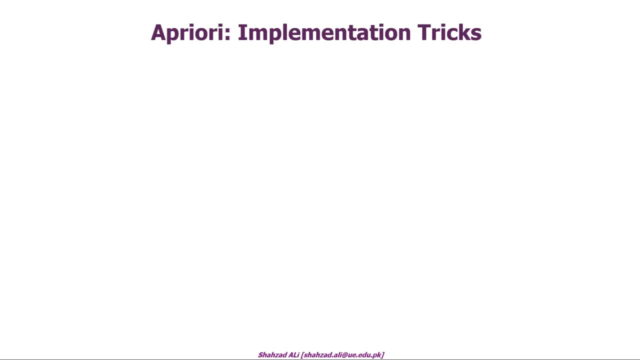 some implementations of a priori algorithm, as, as we discussed in our previous example of a priori principle. we have discussed the self join and pruning concept, so the concrete implementation of this a priori principle involved two steps: the self join and pruning. self joining goes like: 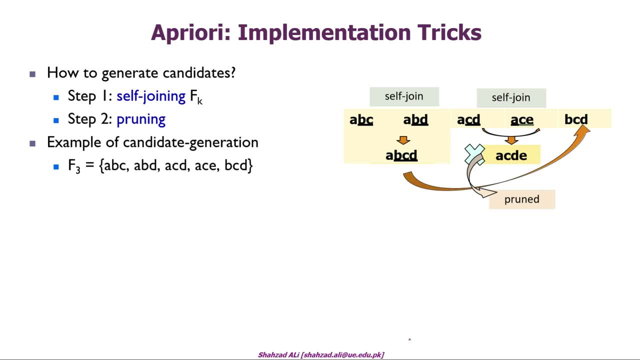 this. okay, we get A, B C and A B D. the first: A, B C and A, B D. the first two are the same, B, C and A and A. in both item sets the first item is same, so 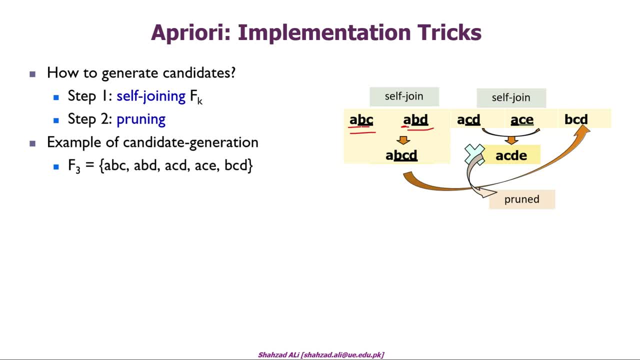 we can generate this self join, generate the candidate set, as the concept of self join means if the items occurs in two different item sets, we only write it one time, so after that we need a pruning process. the pruning is pretty simple before you count against the set of 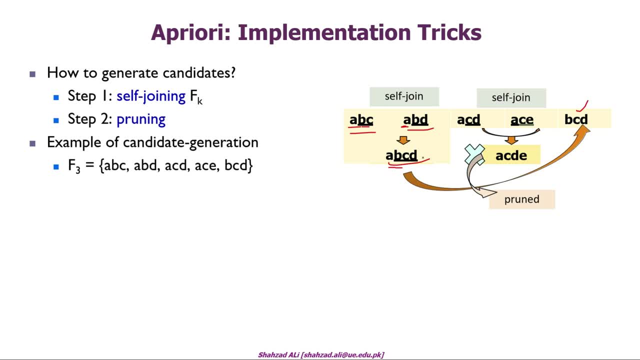 length 3, so we can consider its superset as the frequent. but from these two item sets of length 3, like A C D and A C E, we get A C, D, E as C D, you know. but 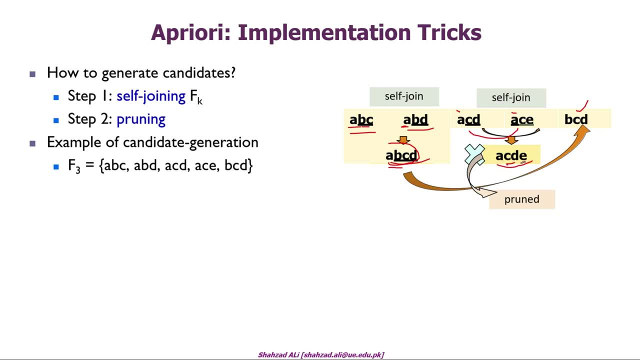 for A C D E. C D is not up there in the frequent item sets, like A C D is the subset of A C D E. so if C D E is not frequent, then its set is. 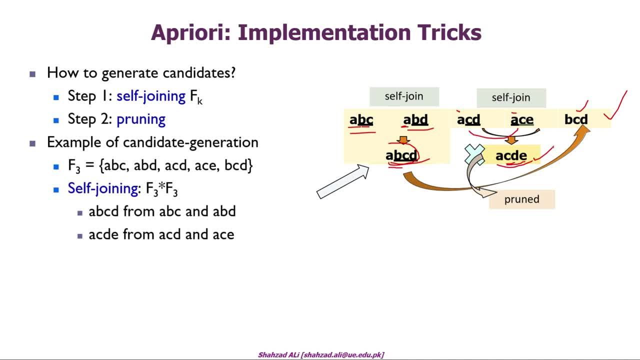 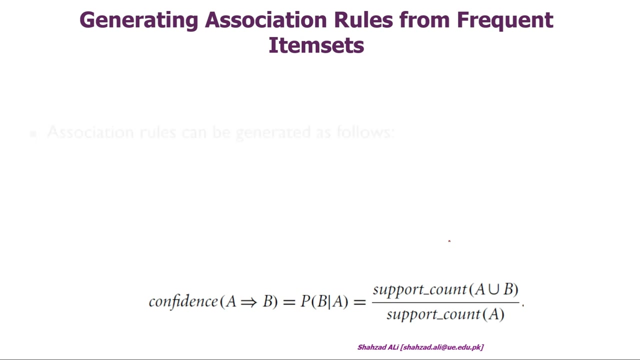 A, C, D E. as you can see in this example, which is discussed in the same way as we have discussed, okay, at the final we get only A, B, C, D, C, D E. so once the frequent item sets from: 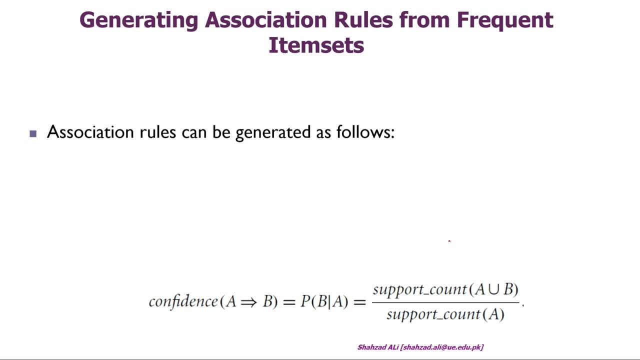 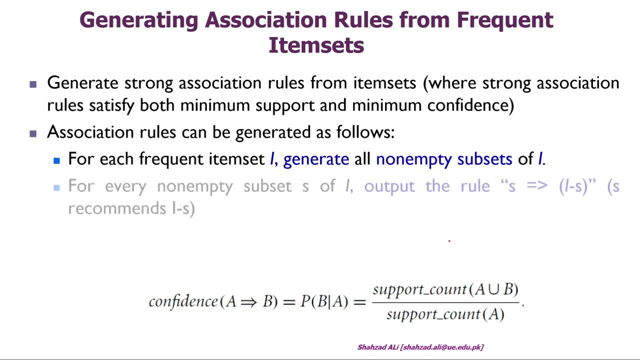 transactional database or from the transactional database D have been found, it is straightforward to generate strong association rules from them, from this equation of this of confidence. for confidence, which we show again here for completeness, the conditional probability is expressed in terms of item sets, spot count. 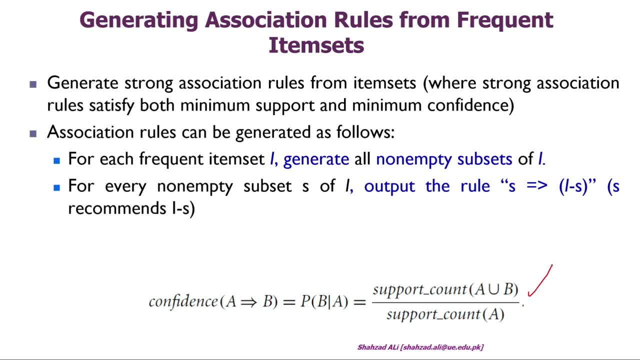 where spot count at CT mark settings at point dot time stop button here written: he next will generate a into set. at present kind of situation We have to consider two things in our mind when we generate association rules from frequent item sets. The first one is: for each frequent item set I generate all known empty subsets of I. And the second step is: for every known empty subset S of item set I output the rule S implies I minus S. You have to keep in mind these two points. 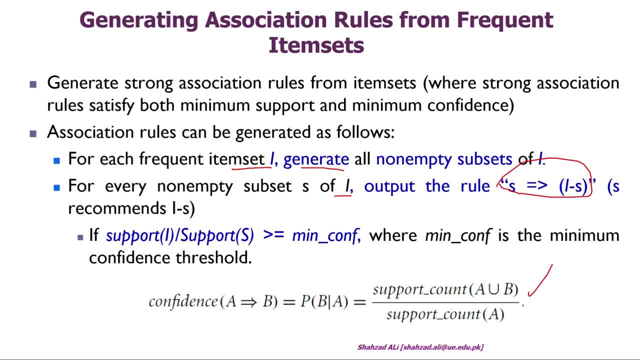 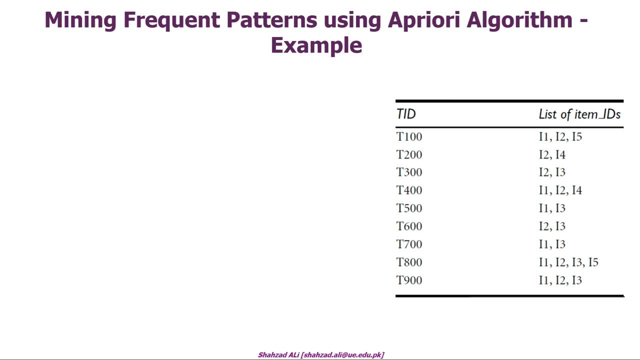 For generating association rules from frequent patterns. So we consider this transactional data and data set which contains nine transactions and each transaction has different number of transactions of different number of items in their respective transactions. So we have to use a priori algorithm for finding frequent item sets. 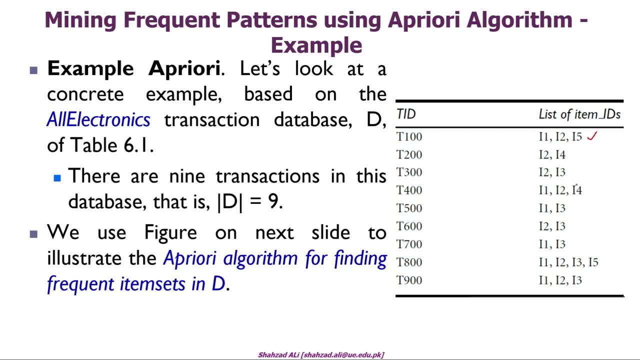 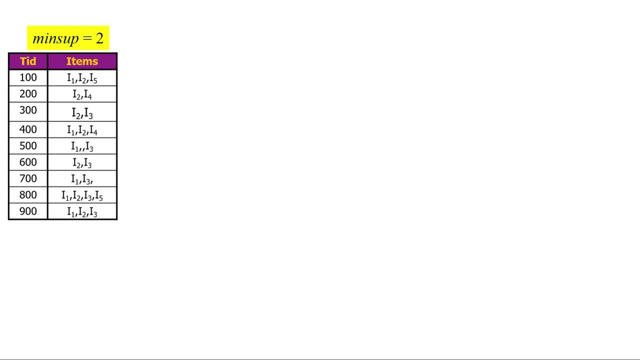 In this transactional data set And then we have to calculate or we have to generate association rules from frequent item sets. So this is the same as we have discussed an example in previous slides. So just we just give you an overview and then directly go into the step of generating association rules from frequent item sets. 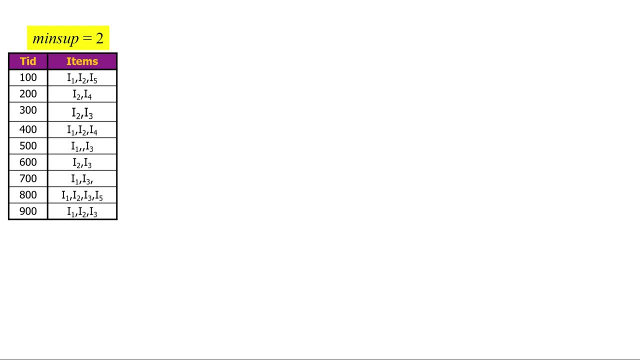 So we have to do our precise calculation of the priority points to set the'm celebratory threshold of the event and the Viv 먹어� And we set the minimum sport�도 to we get these item set S Candidate one itemsVS. 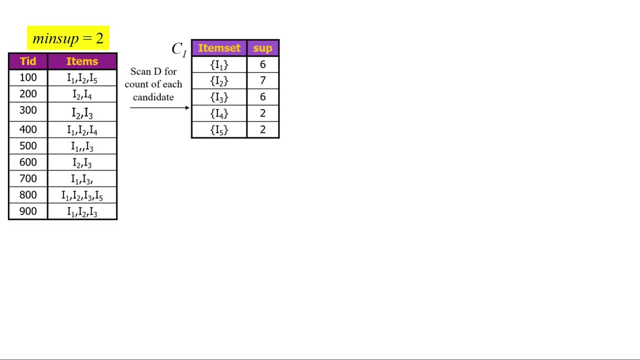 Sort count is six, seven, six, two and two respectively. So from this candidate item setoff, Len't one, we can generate alliances And we can start to generate еще one. we can generate frequent item sets of length two, oh sorry, of length one. so as these all item 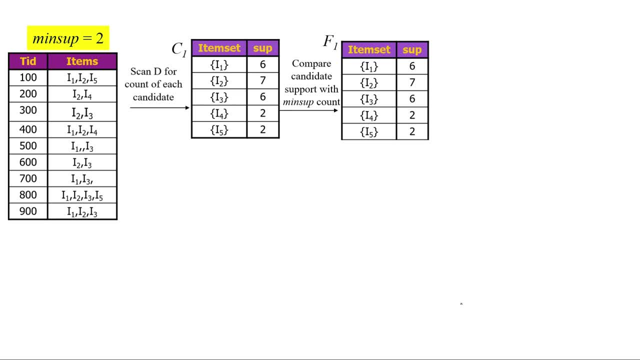 sets fulfill the minimum support threshold value. so that's why these all item sets are frequent one item sets. so from these frequent one item sets we generate candidate item sets of length two as i1, i2, i1, i3, i1, i4 and i1, i5. similarly for i1, i- sorry for i1, i2, i3, i2, i4, i2, i5 and similarly for. 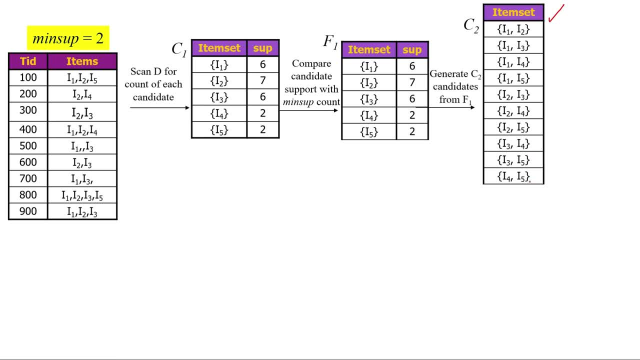 i3, i4, i3, i5 and i4 and i5. these are candidate item sets of length two. then we again go against the database and calculate their support count. as you can see, i1 and i2 occurs four times in the database: i1, i2, 1. 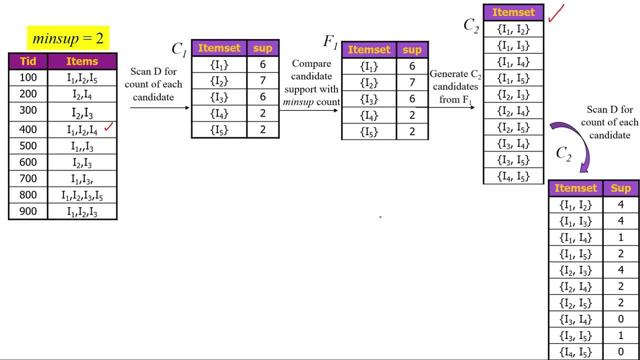 sorry, i1 and i2, i1 and i2, 2, i1, i2, i1, i2. so i1 and i2 both occurs together in this transaction database four times. similarly, for other item sets you can calculate. as you can see, we check i3 and i4, i3, i4, i3, i4. there is not even a single transaction in which these both items. 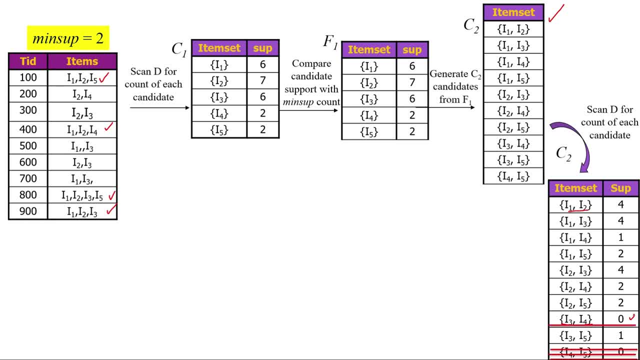 occur together, so their sport count is zero. so that's why we discard the item sets that are below the minimum sport value. so our frequent two item set, or frequent item sets of length two, will be this, which contains i1, i2 or with the sport count of four, i1, i3, with sport count of: 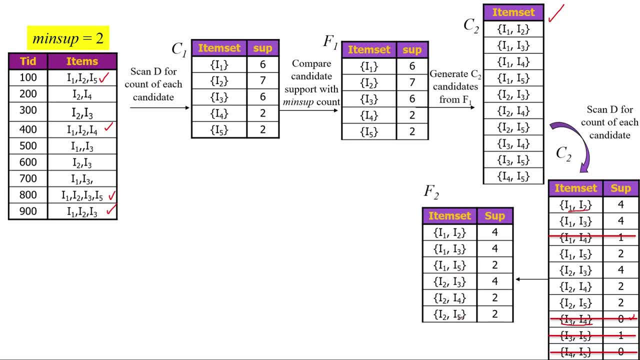 four: i1, i5, i2, i3 and so on. so from this we can calculate candidate item sets of length three. similarly, you can do this as we can, as we have done in our previous example. this is our frequent item set. sorry, candidate item set of length two, with their sport count. 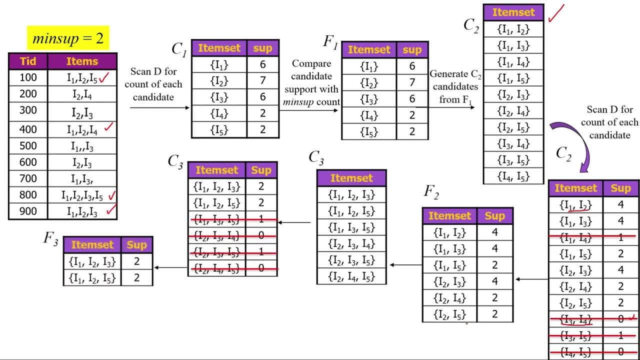 and from this we can generate frequent patterns of length three and their sport count is two and two. so from this frequent three item set we can get candidate item set of length four and the. as this candidate item set sport count is only one because i2, i3, i4 and i1 occurs only once and which is below the our minimum sport. 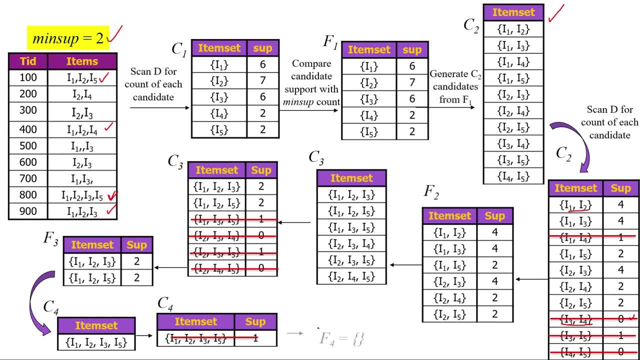 threshold. so that's why the frequent pattern of length four is an empty set. so we only get two frequent item sets of length three, which is i1, i2, i3 with the sport count of two, i1, i2 and i5 with Dise than it means in three. 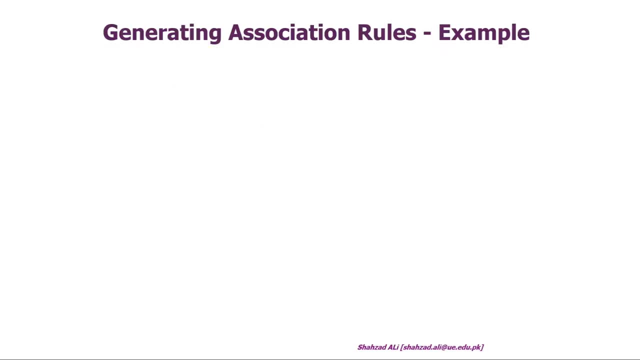 gets below. so for student sorts is very simple. so we use these frequent item sets in order to generate frequent items, in order to generate association rules. so according to the rule of generating association rules, as we have already discussed that, we have to generate sub patterns of the frequent item set. so 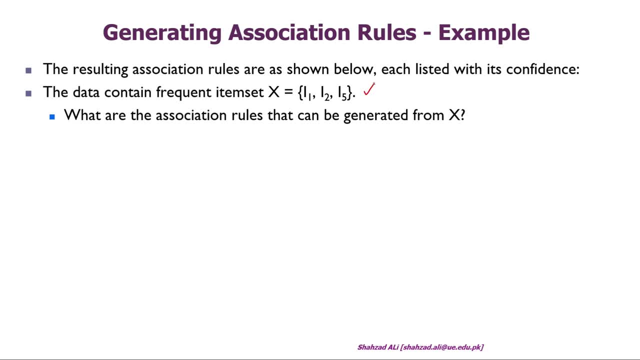 suppose we have considered this frequent item set, which is i1, i2 and i5. so what are the association rules that can be generated for frequent items from this frequent item set? so the non-empty subsets of this frequent item set are i1, i2, i1, i5, i2, i5, i1 alone, i2 alone and i5 alone. so as you can see, uh, if you remember this, uh, sorry. 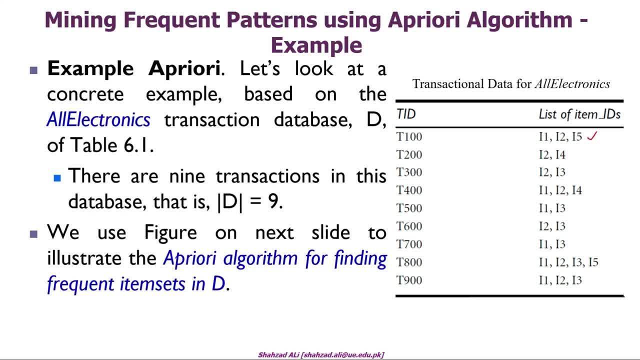 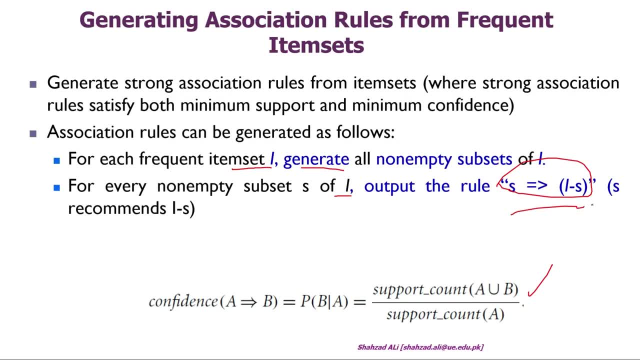 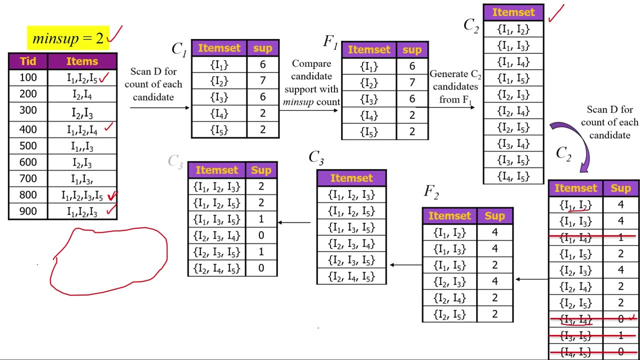 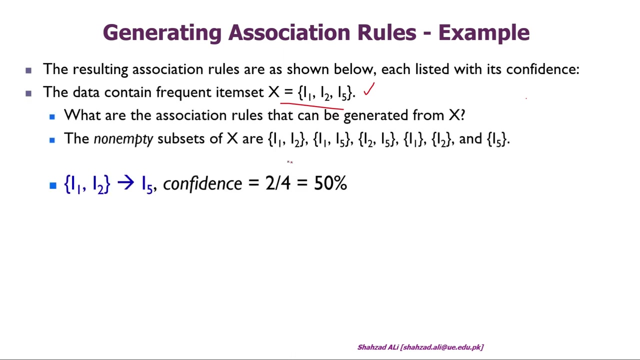 if you remember this principle that you have to generate s implies i minus s association rules. so let's go back into the slide. so, for this subset, this is our subset and this is our item set. i frequent item set i. so this is s and this is our. 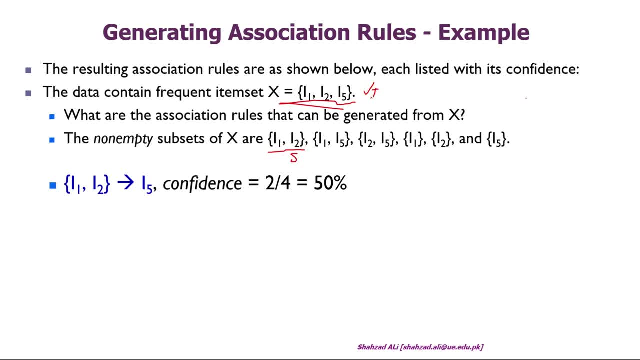 i. so how can we generate? association rule s implies i minus s, so i minus s, we get i5. similarly i1, i5. i5, which implies i2. similarly for i2. i5 remaining part is i1. similarly for i1: the remaining or the. 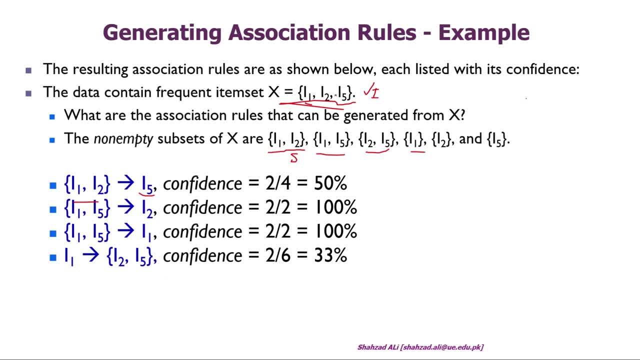 difference of si minus s is i2, i5 and similarly for other two non-empty subsets. so how we can calculate this confidence? so we have to go back into the database. like you can verify these calculations from the transactional database. that means the confidence and the support of these two. 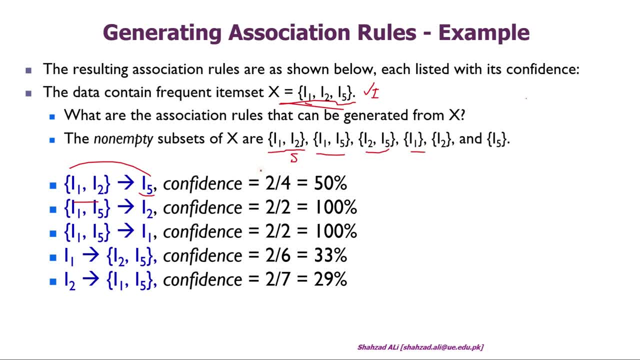 all these three items is two. that means i1, i2 and i5. all three items occur together in the database only two times. however, the support of this part- that means the i1 and i2- occurs four times, so that's why the confidence for this rule is 50 percent.